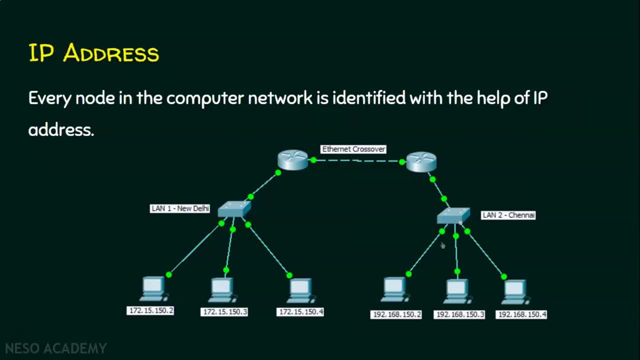 and if I place this computer in the local area network of Chennai and I want this newcomer to participate in the local area network, which is in Chennai, I can simply remove this IP address and I can assign an IP address in this range. For example, this computer is assigned with 192.168.150.2.. 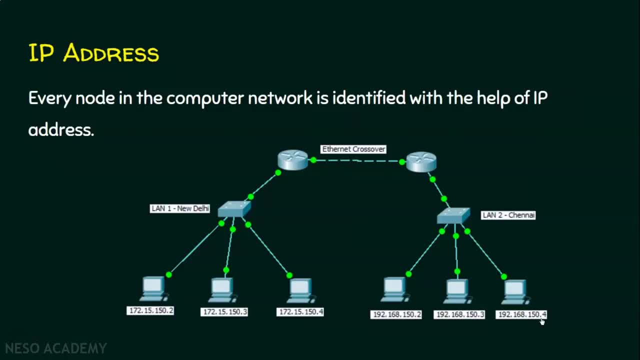 And this is with 150.3.. And this is with 150.3.. And this is with 150.4.. So what I can give, I can take this computer and I can place it here and I can assign it as 192.168.150.5.. 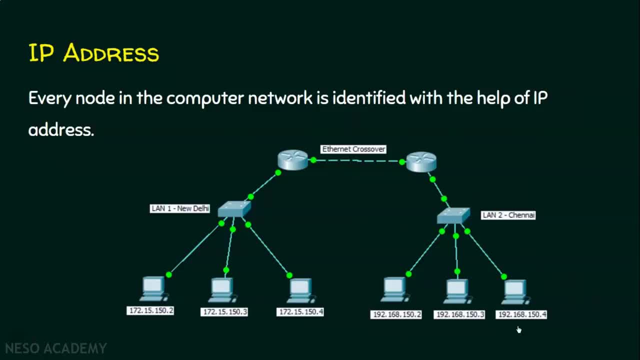 And thereby we can make this newcomer to participate in the local area network. Since this IP addresses can be changed based on the logic or the location, we call IP addresses as logical address, And that is what I have mentioned here. So IP addresses are logical addresses. 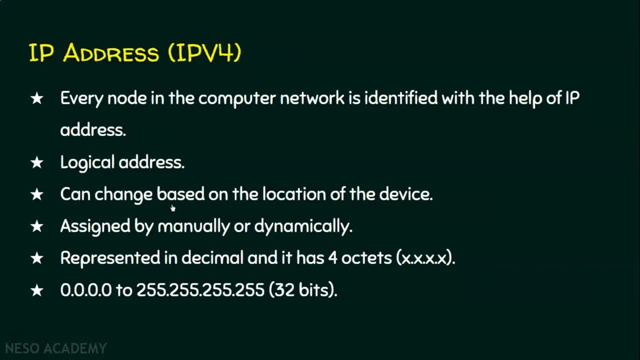 So IP addresses are logical addresses, Because we can change the IP address based on the location of the device And we can assign this IP address manually or even dynamically. We will talk about this point in the network layer, part Time being, you just understand. 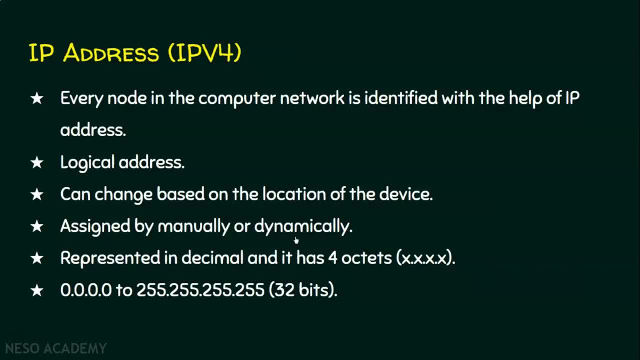 IP addresses can be assigned manually or even dynamically. An IPv4, addresses are represented in decimal and it has four octets. It means four parts Say xxxx, And each of this x takes a value between 0 and 255. 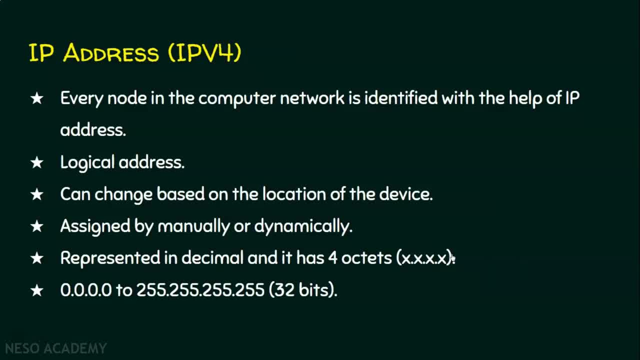 So this x can be between 0 and 255.. Likewise, all the x can be between 0 and 255.. So the starting IP address will be 0.0.0.0 to 255.255.255.255.. 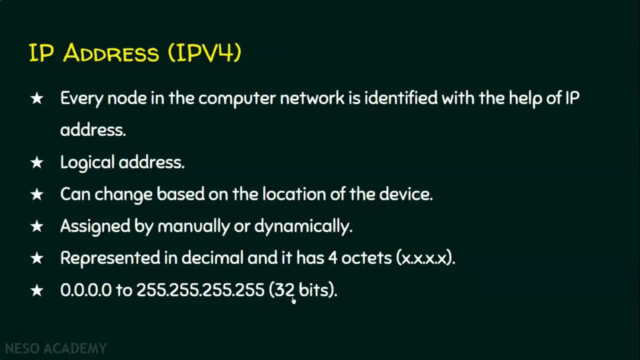 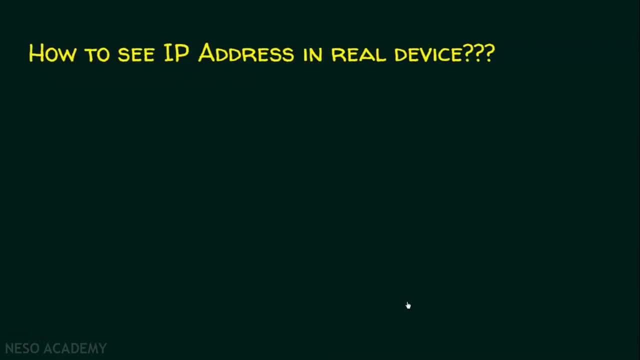 And the total number of bits in every IP address will be 32 bits. We will now see how to see the IP address. Let's first see an IP address in real device. To view the IP address in real device, click the start menu. 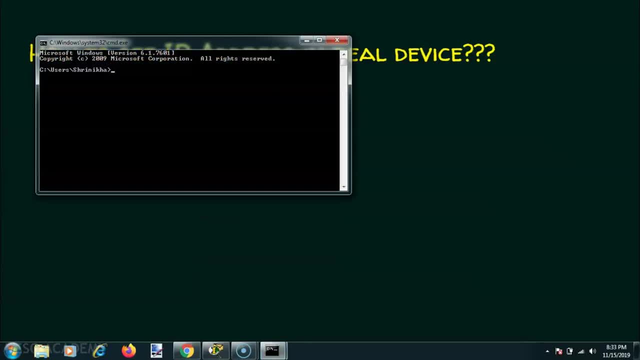 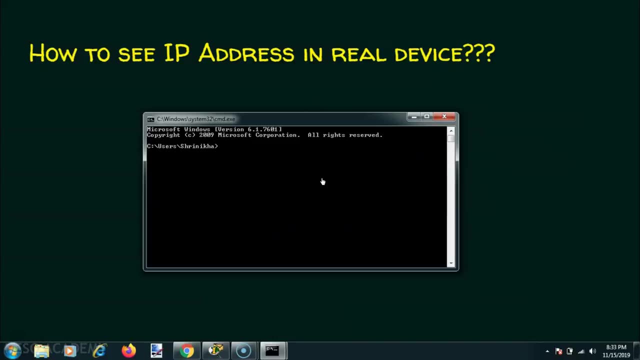 type cnd and give enter. When you give cmd and press enter, you will be given up with the command prompt. This is the command prompt of the Windows operating system that I am using And it can execute all the commands, whatever I give. 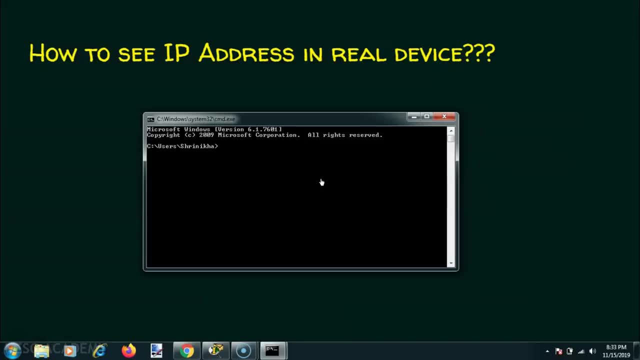 Here I am intended to find the IP address of this computer. To know the IP address of this computer I have to give the command ipconfig. When I give ipconfig in the command prompt, it gives the IP address of this computer. 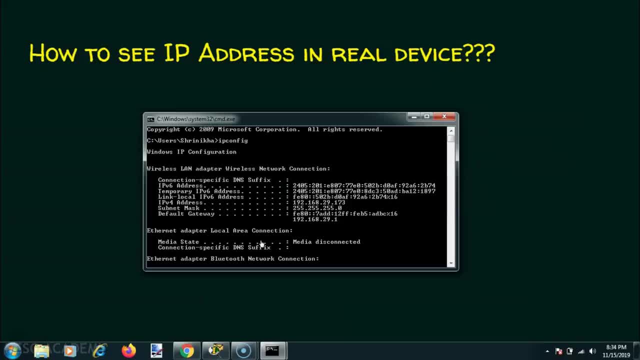 If you observe, I am not using Ethernet based local area network Because I have connected my computer using Wi-Fi And that is why it is showing wireless LAN with certain properties. If you observe, here IPv4 address is shown And this is the IP address of this computer. 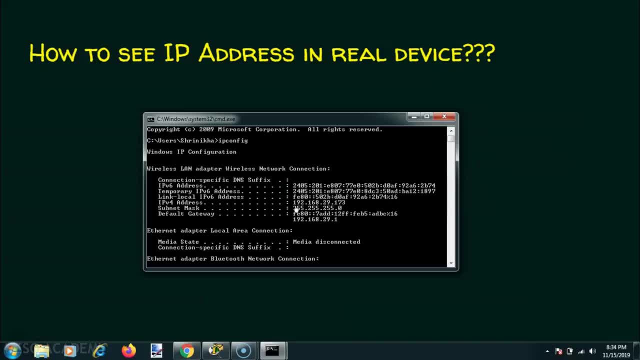 And any data goes from this computer uses this as the IP address For identification purpose. So the IP address of this computer is 192.168.29.173.. So far we have seen how to see IP address in real device. There is an interesting activity for you. 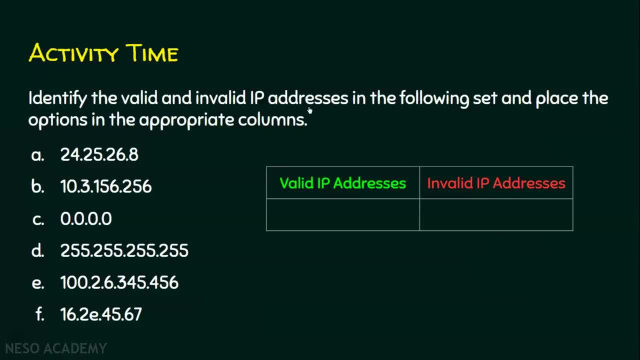 We are required to identify the valid and invalid IP addresses in the following set. So set of IP addresses are given and we are required to identify valid and invalid IP addresses And place the options in the appropriate columns. And there are two columns given. 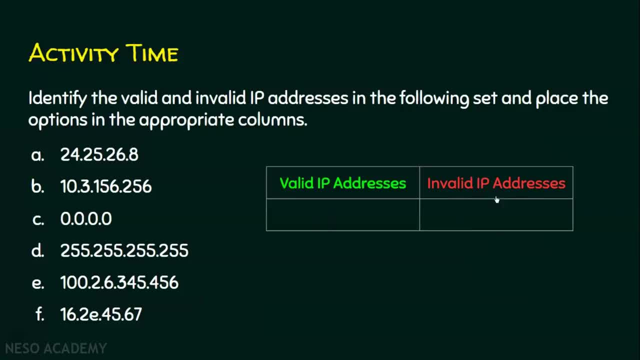 One is the column for valid IP addresses, another one is for invalid IP addresses. Suppose: if you find A is a valid IP address, mark it as A here, And if you find B is an invalid IP address, mark B here, And you should know why they are valid and why they are invalid. 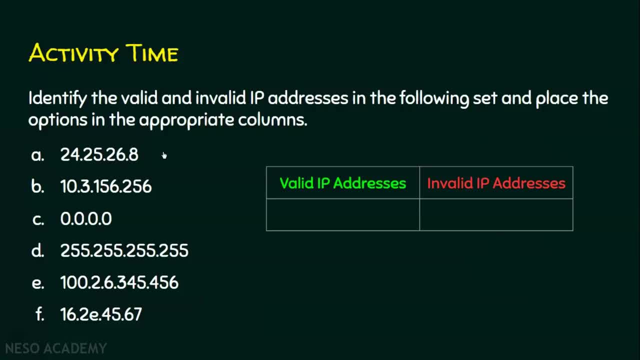 Please pause this video for a while and make a note of this answer against the column, If you are done. compare your answer with the answer that I am depicting. So the valid IP addresses are A, C and D and the invalid IP addresses are B, E and F. 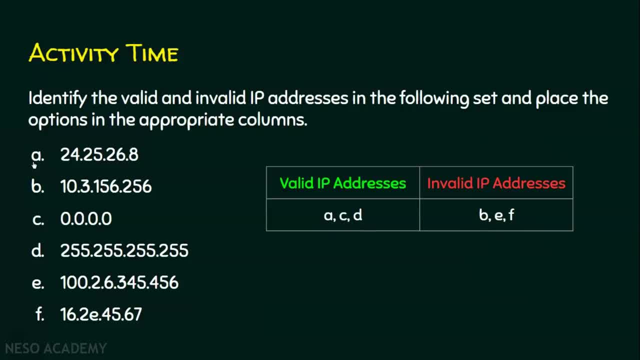 Now we will see why they are valid and why these are invalid. A is a valid IP address because it should have four octets and of course, this is having four octets- One, two, three and four- and each octet is between 0 and 255. 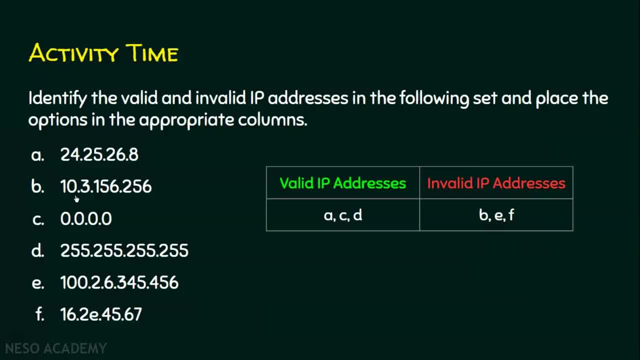 Yes, A is a valid IP address And B is not a valid IP address, Though it has four octets: one, two, three and four. fourth octet is invalid because any octet should be between 0 and 255..